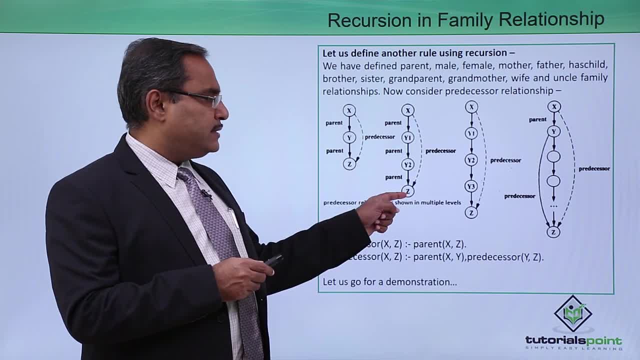 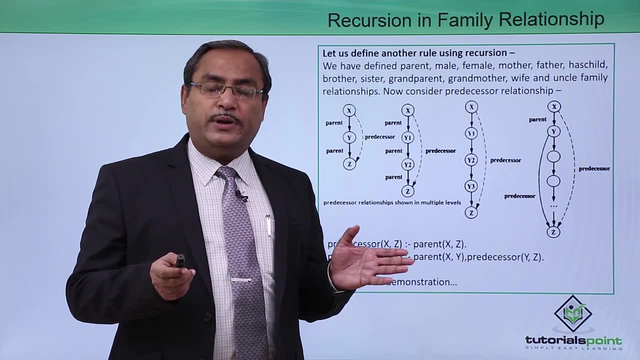 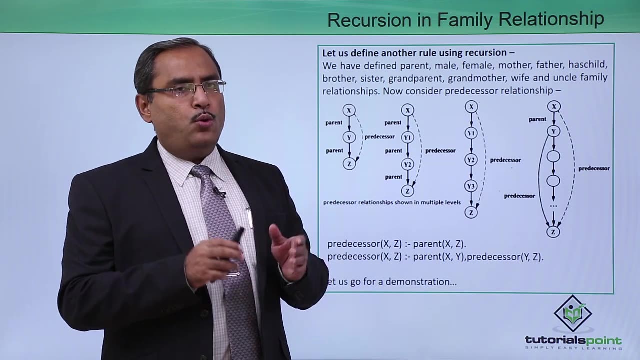 parent of z, then x can be called as a predecessor of z. In this way you can also move one level up. but for how many levels we can write in this way? So that is why, for n number of levels, we must be using some technique with the help of which we can define predecessor. 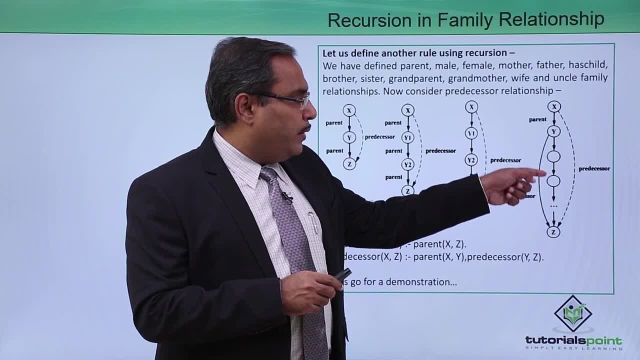 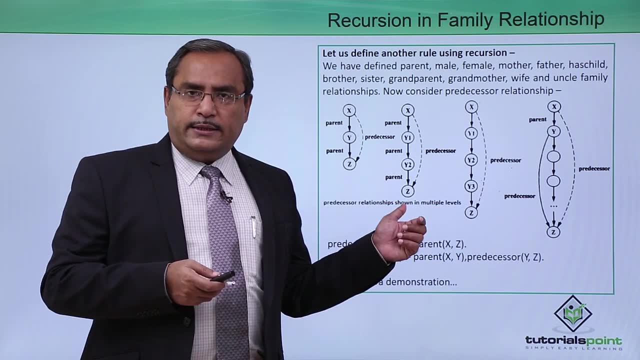 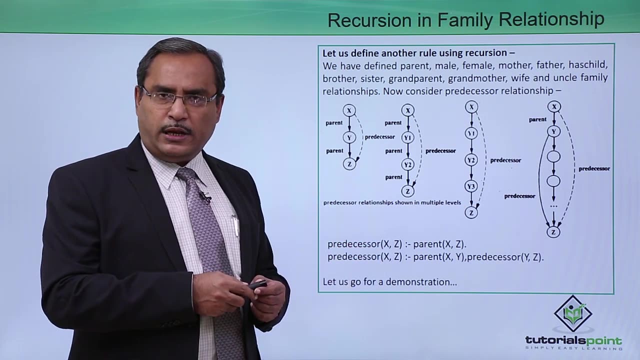 of a person. So here this is another way. So here we are moving up n, level up in this case. So how to write it in the prologue clause? We can write it in this way: Predecessor x, comma z. here x and z are written in the capital letters. that means they are variables. 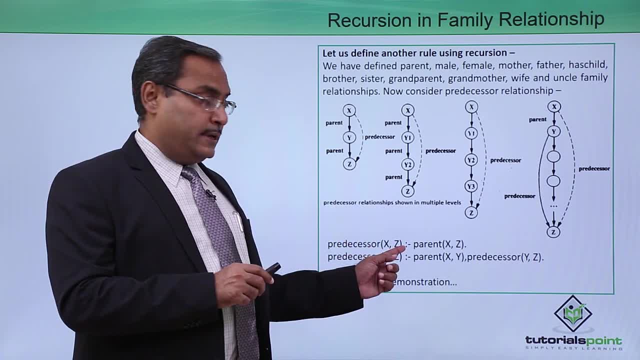 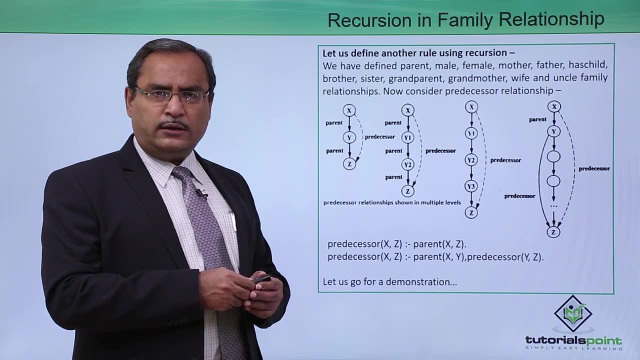 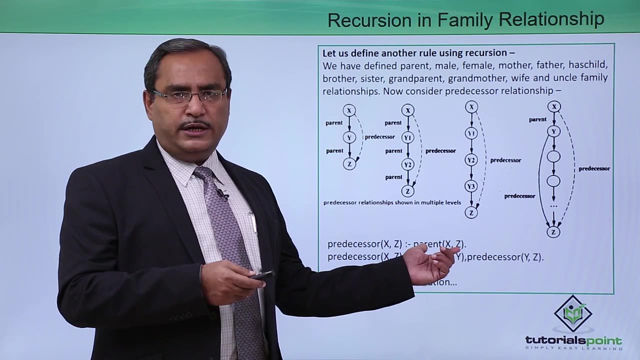 So predecessor x, comma z, if parent x z, so that is, that will get satisfied by our given facts at this point. So here we know that clauses have got divided into facts and rules. So parent x z- we are having some facts given from there. it will get instantiated. So predecessor x z can. 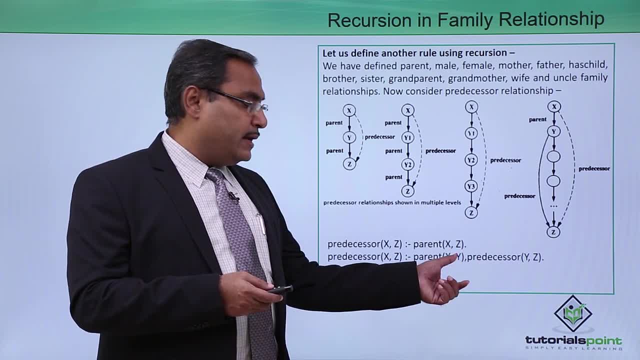 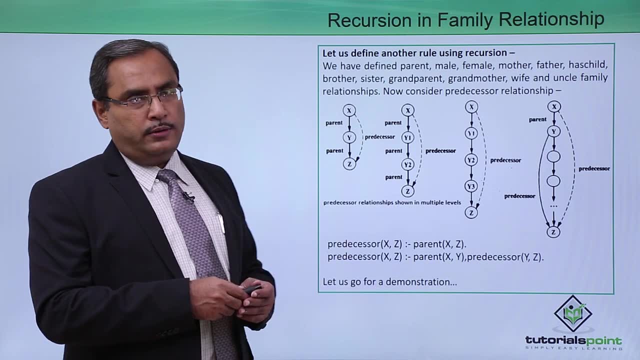 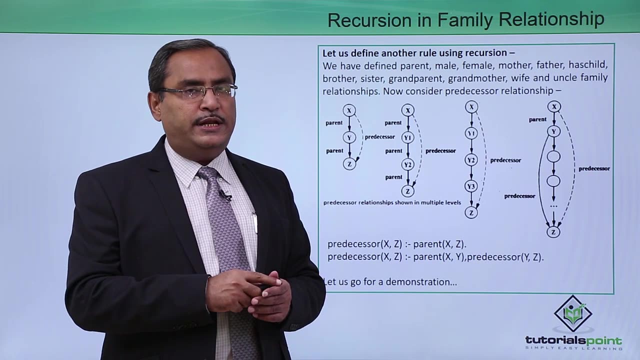 also be written as if parent x- y and predecessor y- z. So here you see, we are using the recursion in our prologue. At this moment you can pause the video and try to write the prologue clauses to define this predecessor relationship. otherwise, demonstration is always for you and please watch the 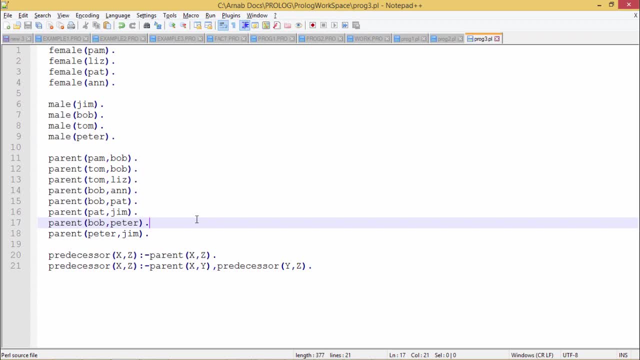 demonstration for the better idea. in this program we have introduced another new clause that is predecessor, so predecessor X comma Z if parent X comma Z, otherwise predecessor X comma Z if parent X comma Y and predecessor Y comma Z. so in this way, in this predecessor clause declaration, where we used to: 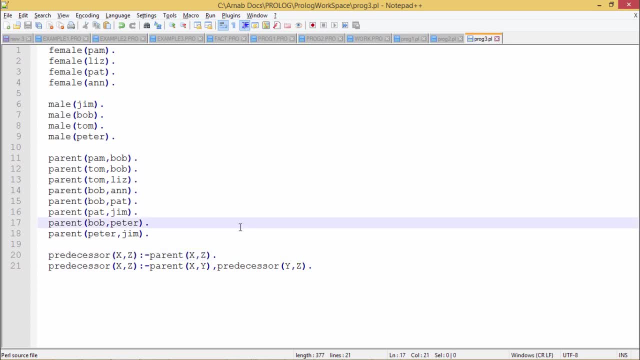 recursion. we know that in case of recursion were having two issues. issue number one is that a recursive algorithm or the recursion should have some case where the algorithm will terminate it. so here this is our base case: an recursive algorithm must have a calling instruction to itself, either directly or 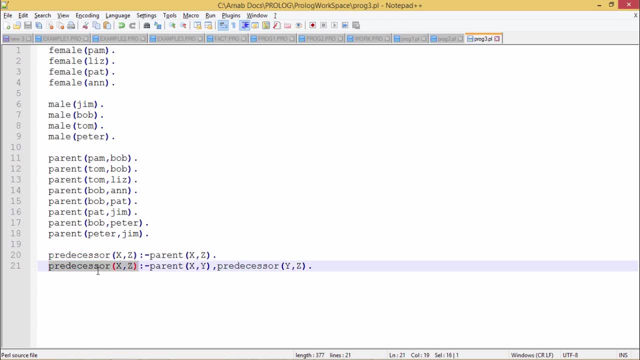 indirectly so, while declaring this predecessor clause Truths which don't line up in class class plan. when you're taking rest of the class, we have clock. we have called this predecessor again, so within the right hand side of the predecessor of this clause declaration. so that's why it is a good example of recursion. 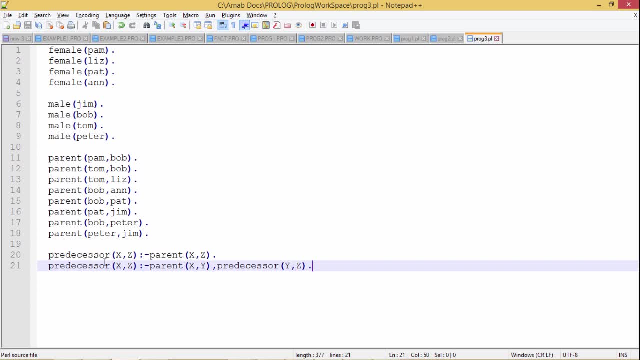 so prologue supports recursion. so predecessor x comma z will be nothing. but if z is one level higher than x, is one level higher than z, then it will work. otherwise we can go for multi-level higher. so that is predecessor x comma z if parent x comma y and predecessor y comma z. so now let me. 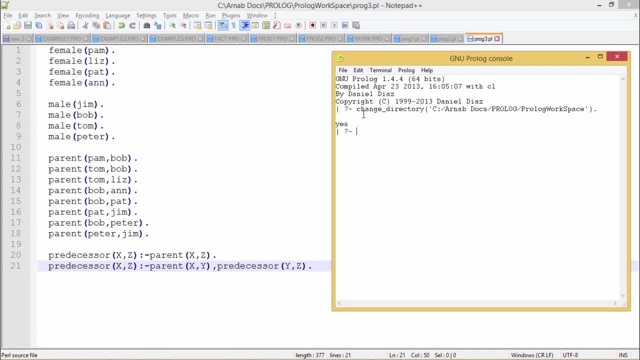 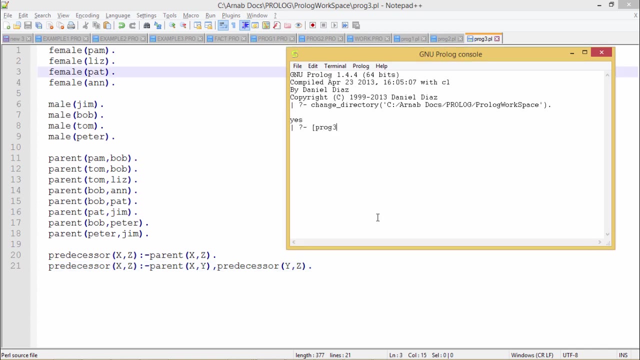 execute my code. so here we have done the change, direct directory accordingly. so under the prolog workspace my program, that is, proc3 dot pl, is deciding. so now let me execute. so it is causing failure. so that's why no answer has come. so if you go for predecessor peter x, 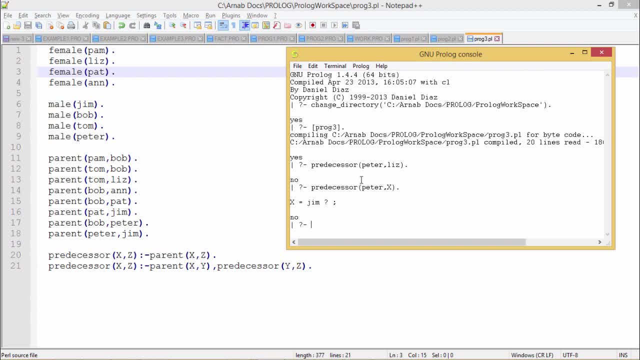 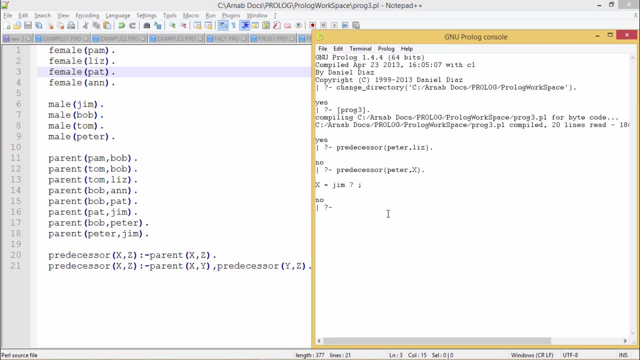 i'm getting this gym as output and there is no other answer. so let me do the tracing of this. so, for the better understanding, let us go for the tracing of this. so we should initiate the debugger press and then we are writing the query. so here you see, at first predecessor. 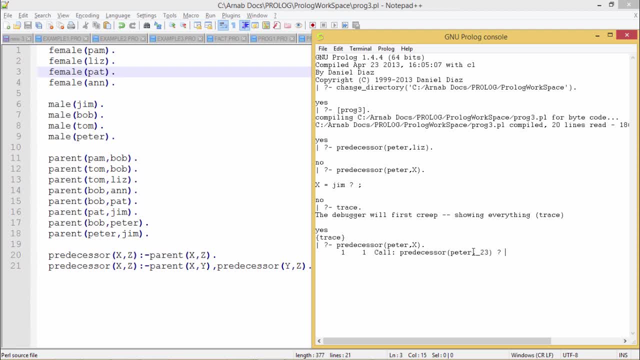 peter and this anonymous variable name, internal variable name, will be there. so at first it is executing this one. so x has got initialized with p peter and this z is being represented by this underscore 23.. so we are pressing enter. so parent peter, underscore 23. so it has been called accordingly. 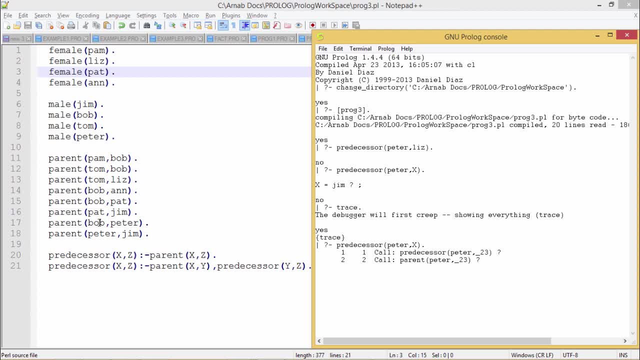 so now it will go for checking whether peter is parent of someone or not. yes, gym is the answer in that case. so pressing enter, so exit. exit means coming out with success, otherwise here the fail will come. so you see: exit peter, parent, peter, comma, gym. so it is coming out with the solution: gym. 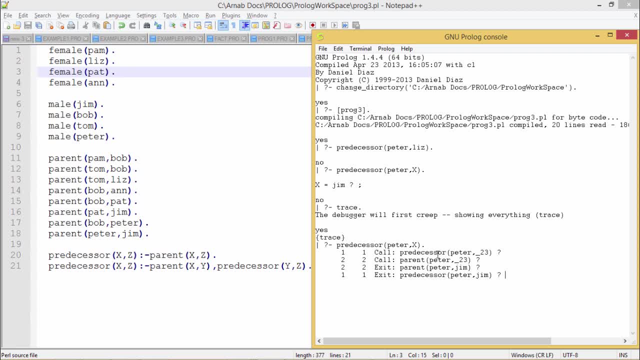 and then exit. predecessor peter comma gym. so here you see, it is one one, so that this particular predecessor, which was called it, has got a success while coming out. so one answer, i have got gym. so now let me go for the next one. so it will go for a predecessor peter gym. in this way because 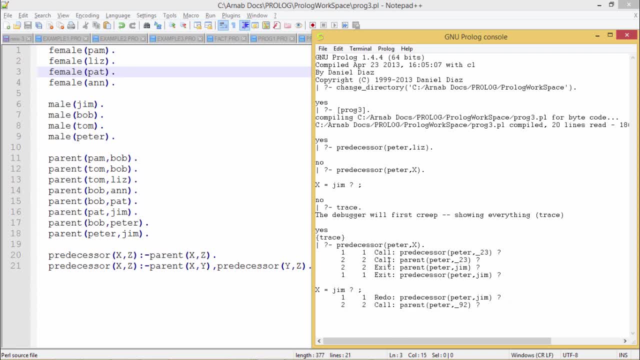 gym. i've got the answer already. so now parent peter this. so parent peter, this y has been represented as underscore 92, so now it will go for parent peter gym. so now it will go for parent peter gym. so it is coming out with the success because this: 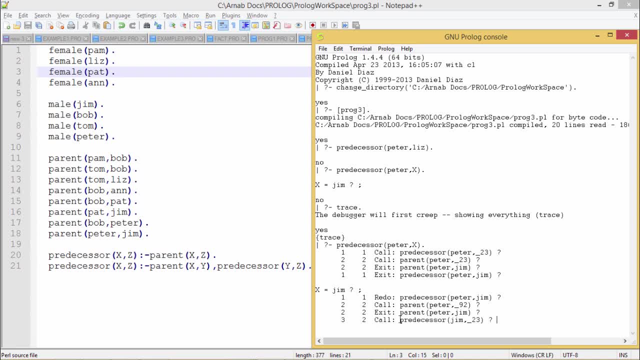 peter gym is there, so parent peter gym. so now it has called to predecessor gym. that is underscore 23. so now it is coming coming down to this. so here it is being called. so again the base case, base condition is getting tested, so it is going for parent gym, underscore 23. but here you see there is no gym here in the first argument. so 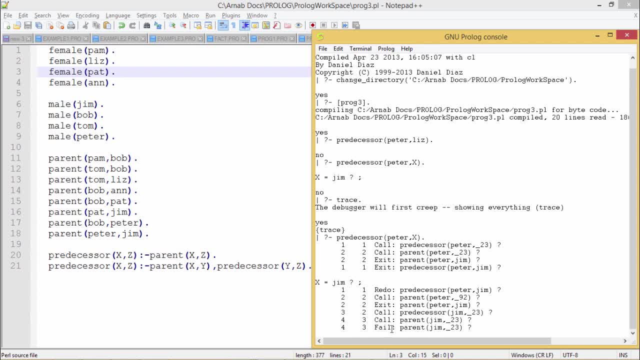 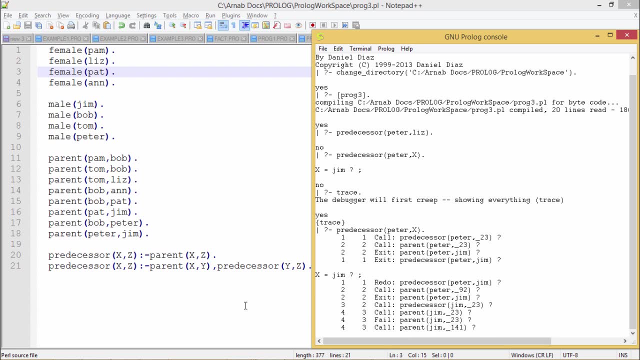 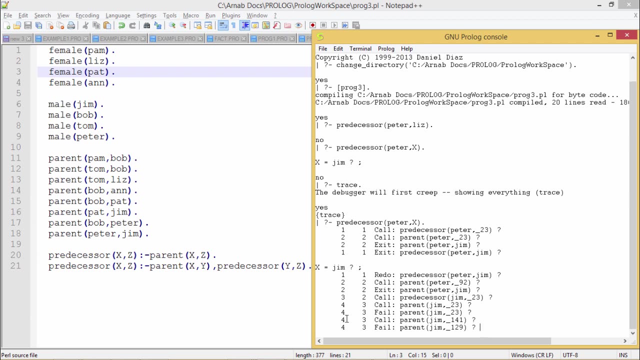 it is coming out with the fail, so that is four: three has been failed. so now this is my parent gym underscore 141. so it is coming down to this: so it is failing. so 4: 3 is failing. that is the 4: 3 call of parent has failed, so it has failed. 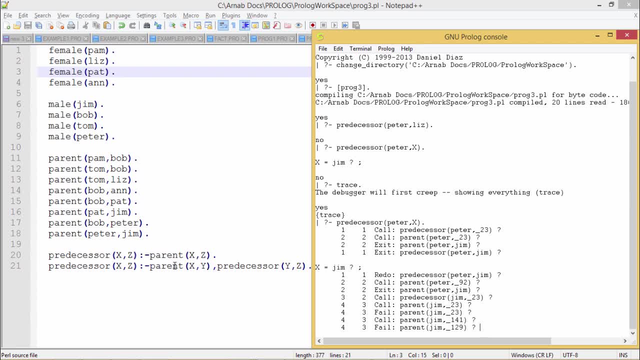 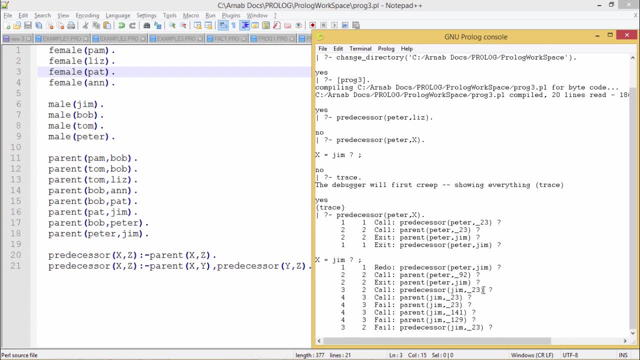 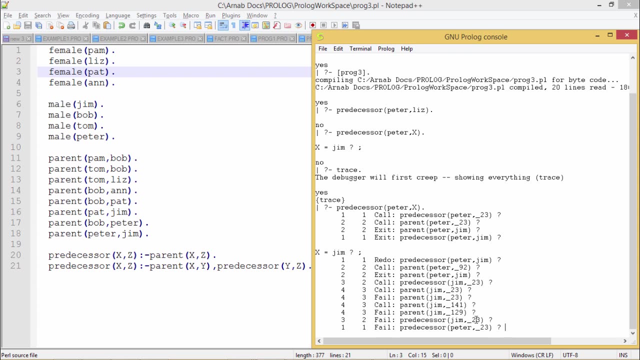 and and condition is there, so there is no need to check this one because this condition has failed. so now it is going for 3: 2. so 3: 2- that is predecessor gym 23- has failed. so this 1: 1- that is predecessor peter gym- has failed. 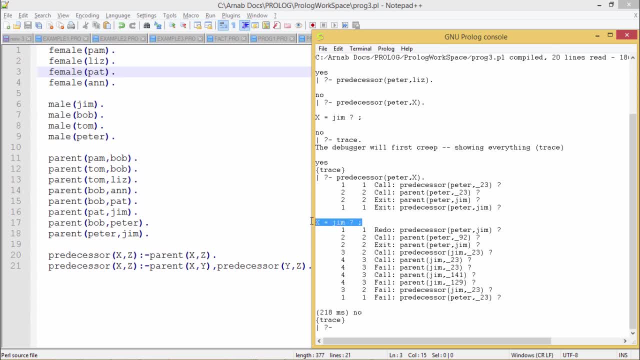 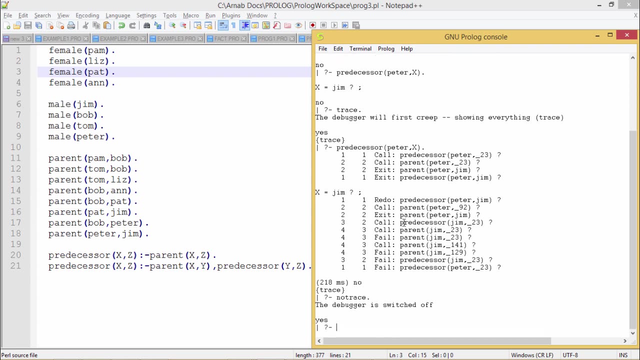 so there is no answer and only one answer, where whatever we got is our x is equal to gym. so in this way the tracing can be done and in this way the outputs can be obtained. so let me type no trace to close the debugger, and now you can execute the same. 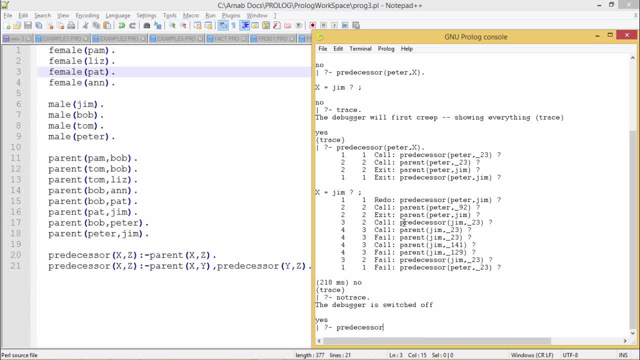 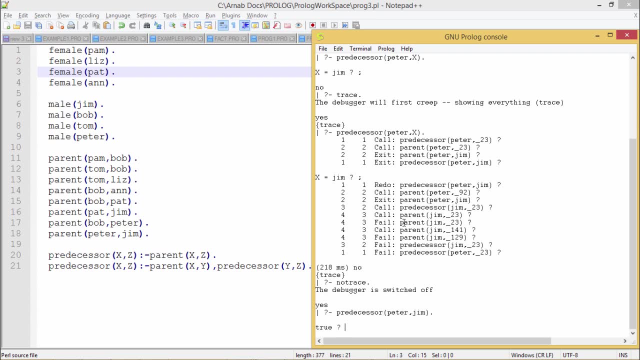 so now we can need the letters x and y. well, in this way, if you, uh, we need love term name, whatever it be, it's going to that um you have, the product name is, and so the result is that you can only string the initial direction now. 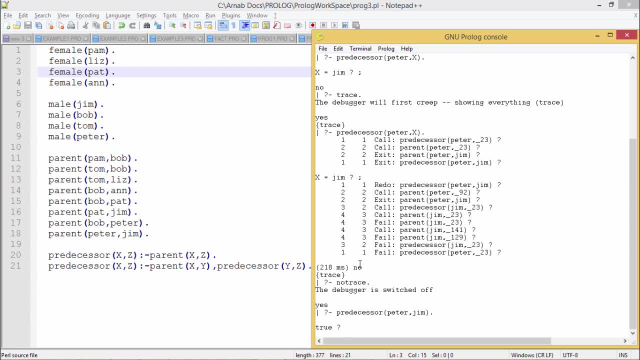 we need the real Hello feature, which is the fromライ delta I only as is not true. so, and that's the way in which you create this- ViewActions helped plot different values. it is very easy, and I'd like to understand the answer to that problem, so let me show you so now. I'm getting the answer as true. so in this way my uh new class, that is predecessor, has been tested with that with tracing and without tracing and all. and write such program at your end and going doing the tracing with other values for x and yx and z here, rather that would not be too hard and problem. so let me pause and read the following words here: Thanks for watching this video.